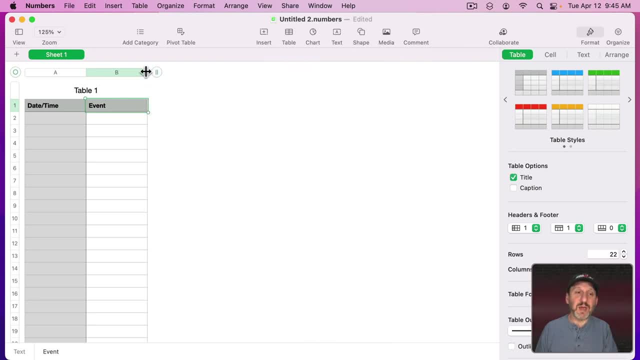 for the second. Then I'll get rid of all the additional columns, Maybe lengthen this column A little bit right there. There's no data in this now, so I'll shrink this as much as I can. I have to have at least one row in here. that's not a header row, So I'll just leave that blank. 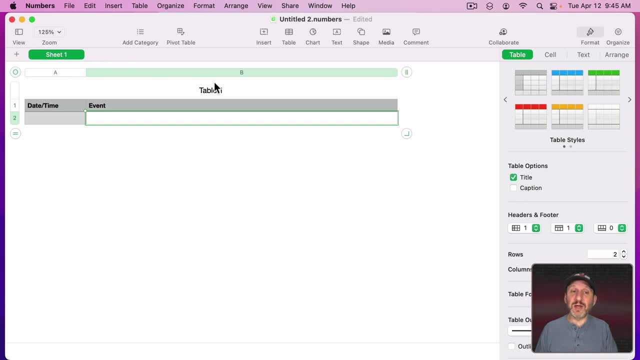 Let's name everything properly. I could leave the name as Sheet 1 and Table 1.. But let's actually give them proper names. I'm just going to double click in here and call this Data. Maybe this is the Data sheet and you have other sheets that show reports and things. The Table here. let's 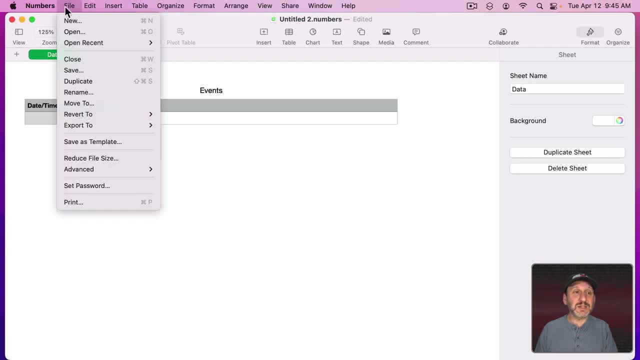 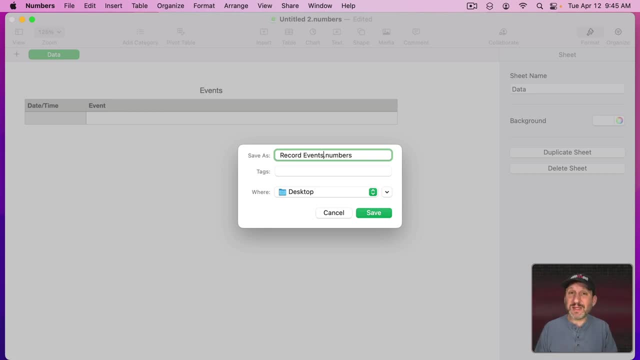 just call that Events. So let's save the document- I'm going to call it Record Events- and just put it on my Desktop. You should probably put it somewhere in your Documents folder, But I'll put it on the Desktop so we can easily see it here. 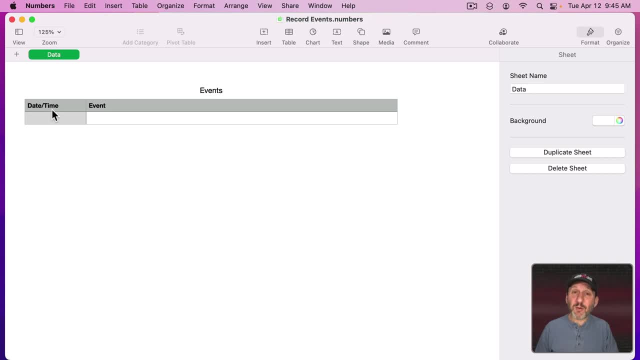 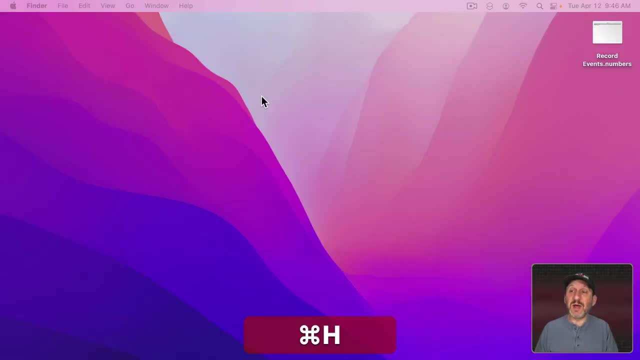 during this tutorial. So I've saved that. So now what would be nice is if I could trigger a shortcut to actually fill in a Date and Time and Event. Let's hide Numbers here for now. We could see the file there. Let's launch the Shortcuts app. I'll create a new shortcut. 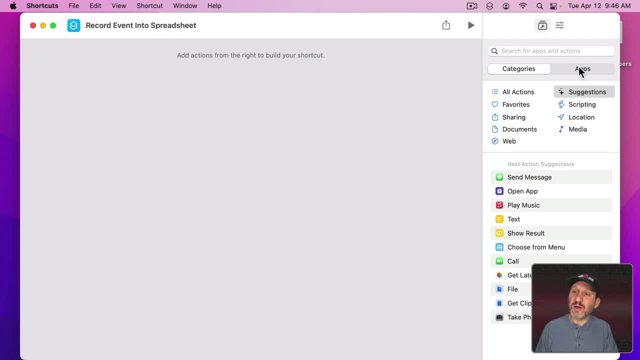 Let's call it Record Event into Spreadsheet. I'm going to search over here under Apps for Numbers. Here I can find three actions that pertain to Numbers. So we've got one here called Add Row to Top or Bottom of a Table, That's. 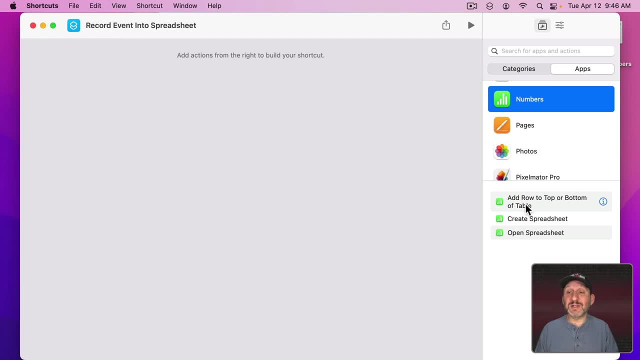 exactly what we want. We don't need to create or open the spreadsheet in advance, We can just go right to this. So I'm going to double click it to add it. Now we've got Add Values to the Bottom. We can do Bottom or Top and then we define a Table Sheet and Document. 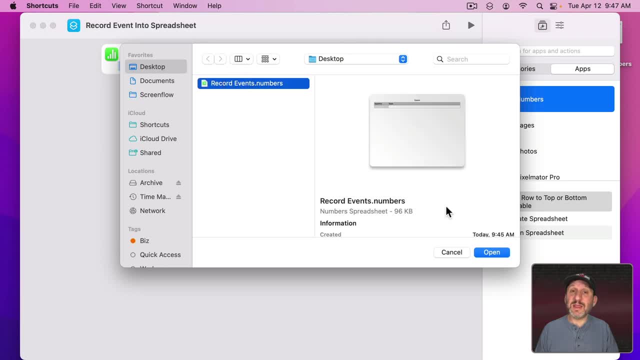 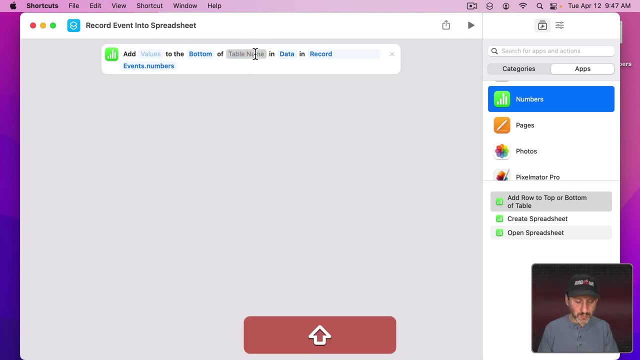 Let's work backwards here. I'll click here and select that document. Great, The sheet name, remember, was Data. The table name was Events. We do want to add to the bottom. Then what do we want to add? Well, we want to add the date. 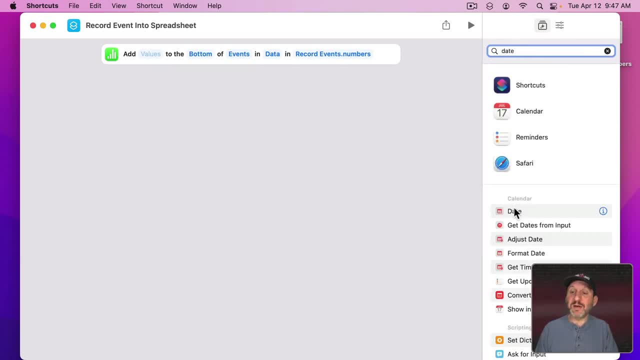 So let's go and search for Date here and there is an action for getting the current date. Let's move that above here. That gets the current date. If we wanted to, we could format the date. Let's put Format underneath Show More and we could select the Date and Time format. 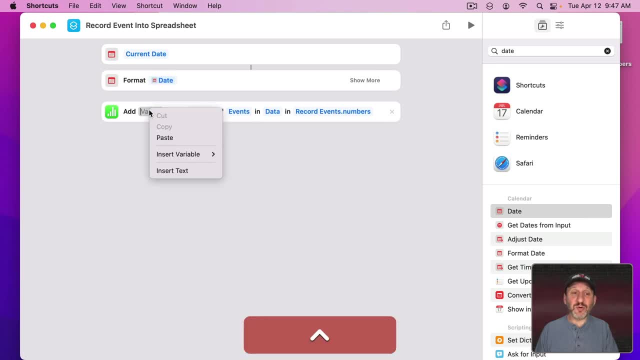 Now let's click here and I'm going to actually Control- click in here and do Insert Variable, Select Variable and select the result of the formatted date. So it takes the current date and time, formats it like we want, and then it's going to use that in what it adds. 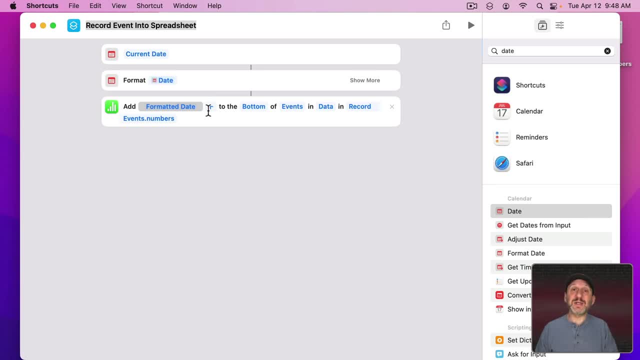 to the table. Now there's also a Plus here that allows us to add more data, So this will add one, one cell. We can use this here to add another cell and continue going, But let's test this out first. So I'm going to go to Settings here and I'm going to pin this in the Menu Bar. 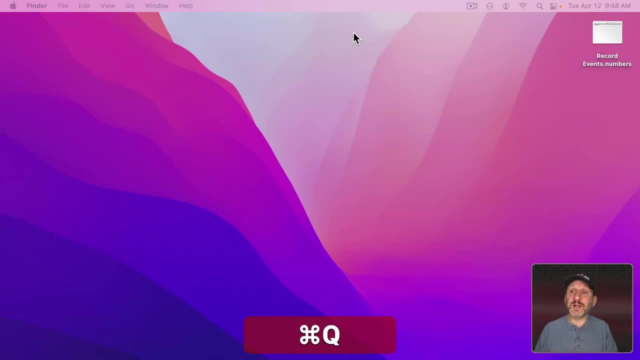 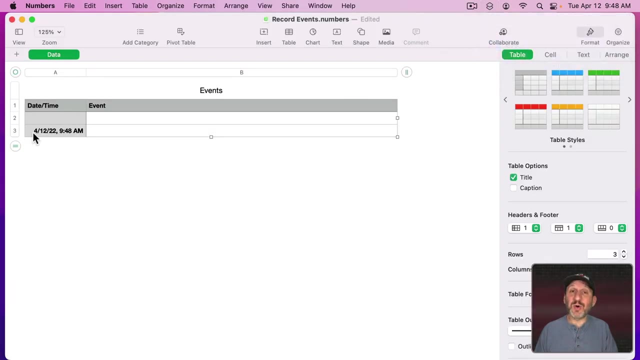 So now we see it right here. Now I can actually Quit Shortcuts. If I were to run this, it's going to open up the spreadsheet and, sure enough, it's going to put the date in that format right here and nothing for Event, because we're only adding that one cell of information here. 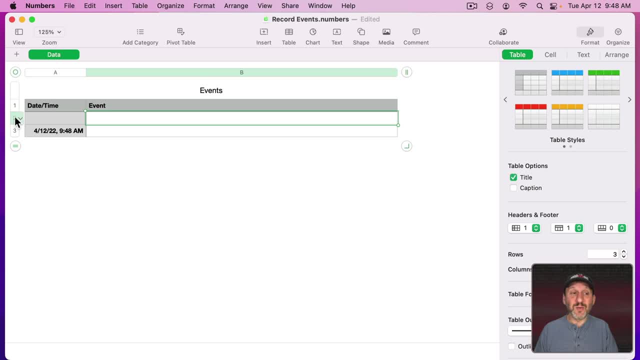 The first time we do this, we're going to end up with a blank line, because we had to have a blank line here in order to keep the table there, So now we can get rid of that. Now, anytime we use this again, whether the spreadsheet is opened or not, it's going to open it and then add something new. 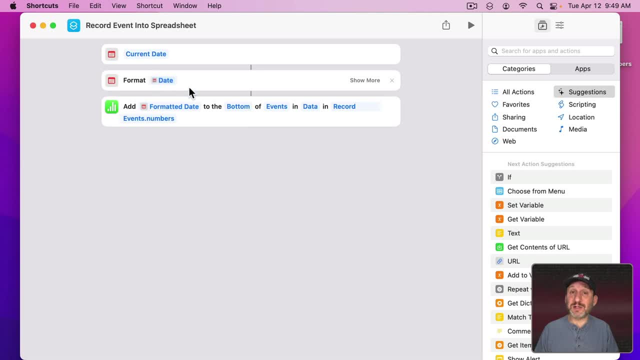 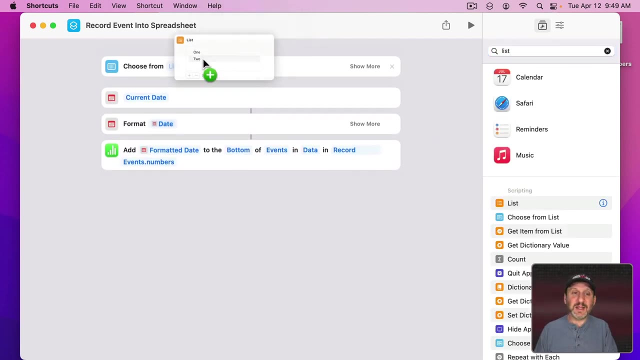 to it. Now, what would be nice is if we can actually record an event as well. So to do that, what we want to do is search for Choose, and there's Choose From List. Let's add that to the beginning here We need a list of items, So I'll search for List and let's add List up above. So we first define. 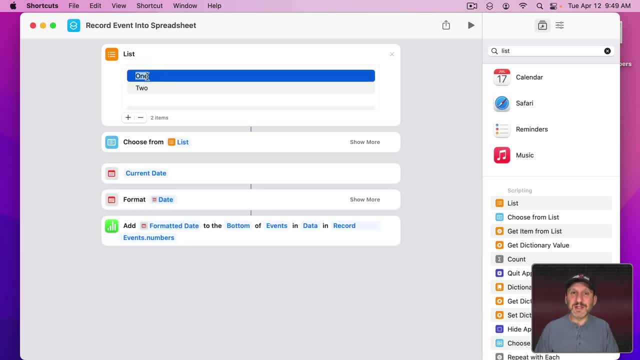 the list. Let's define a bunch of events here. I'll just create some sample ones. This creates the list. We see, it says Choose From and it automatically selects the list, and so it was right before it. If not, we could have clicked here and then selected List as the input. 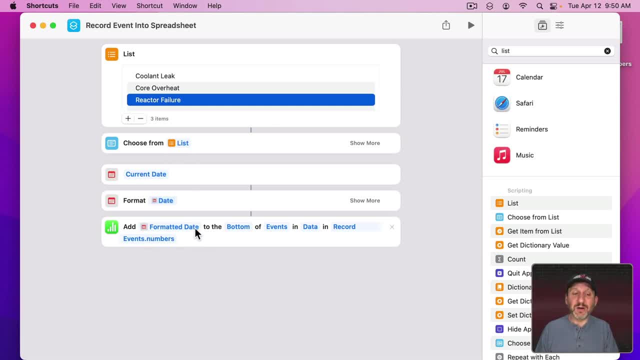 Now we get that data here. We want to add it here. So where did that Plus button go? Unfortunately, that Plus button is gone. I'm going to control it. I'm going to control it. I'm going to control and click on it and Clear to clear that out. Click again to add value. So the first value I want. 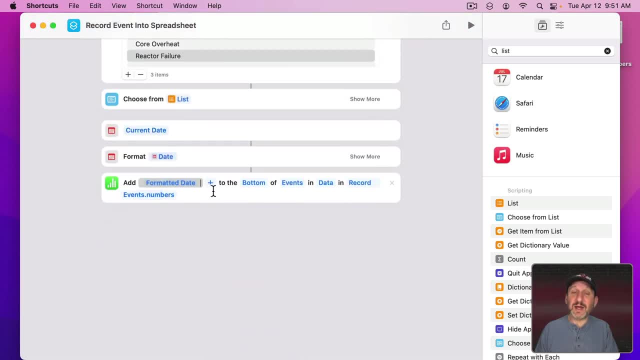 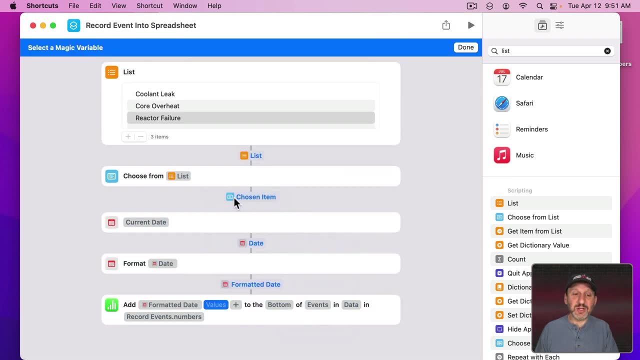 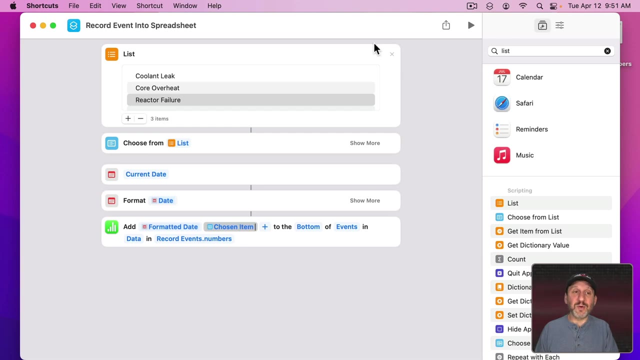 Insert Variable, Select and get the formatted date. Now that Plus button is back, Click that Control. Click Insert Variable, Select Variable and get the chosen item here. So now I want you to add two things to that row: The formatted date and the chosen item. So I'll quit Shortcuts and 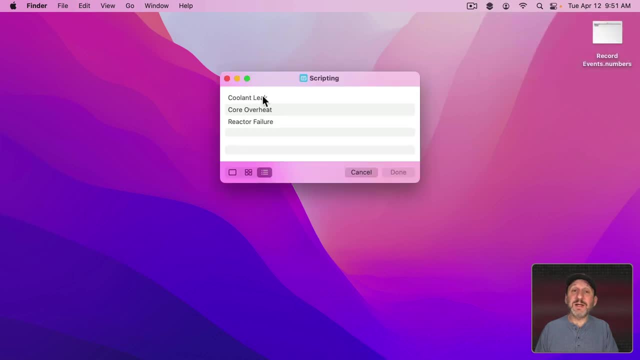 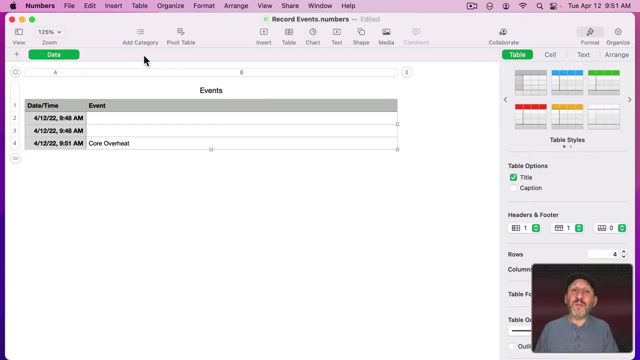 I'll run it again. You can see it comes up with this nice list. I can select one and click Done, or just double click that item. It will open up the spreadsheet and add that here. So you can add one or many more items to a spreadsheet row, always creating a new row there. It would be nice if it didn't. 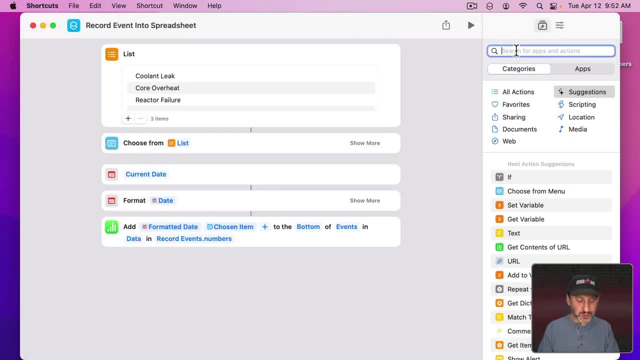 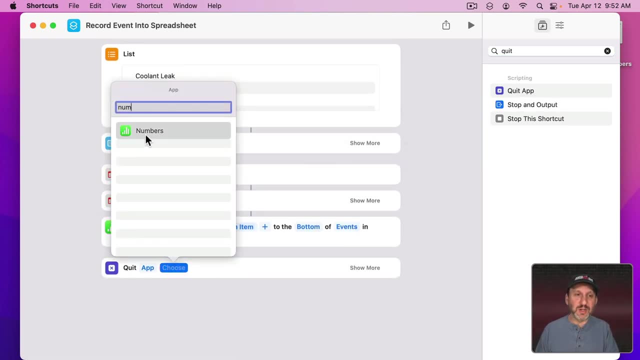 leave us sitting here in Numbers. You can kind of add that to the shortcut. If I search for Quit, I can do Quit App. Choose the app, Search for Numbers. What I find is that it doesn't quite work, unless you had to wait, because 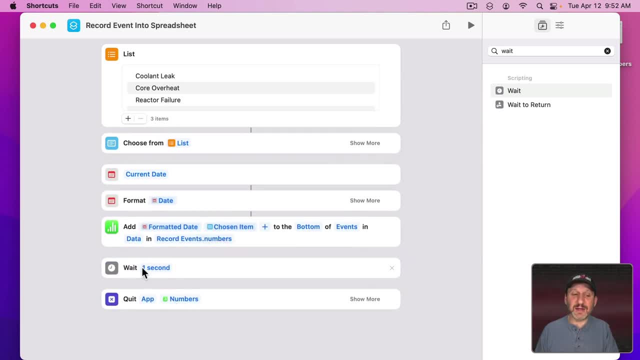 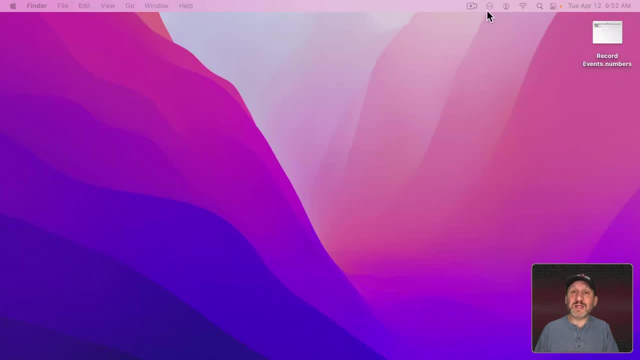 it's still working on this when it tries to execute that, and so it won't quit. So you have to wait for, say, three seconds here, which gives us time to review the entry. So now, if I wanted to add an event, I could trigger it like that: select one, you could see it adds it there. 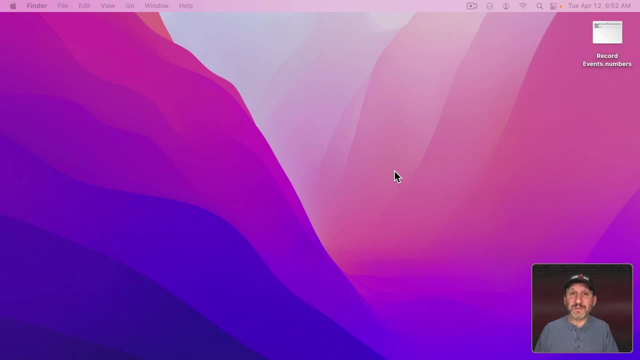 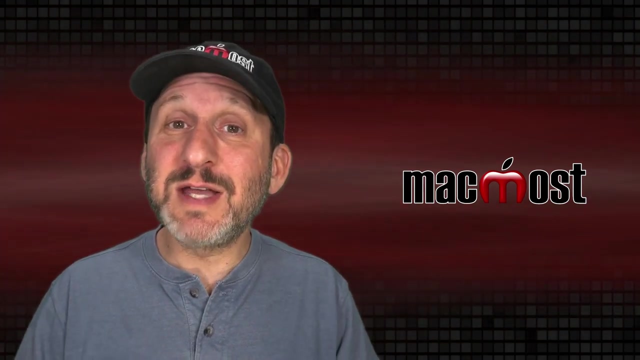 and a few seconds later it quits Numbers. So you could probably see all sorts of things. I'm going to click on the button and click Go. You can record all sorts of data into a table in a spreadsheet. The spreadsheet doesn't just have to be that table. It could be a complex spreadsheet. You're just adding a row to a 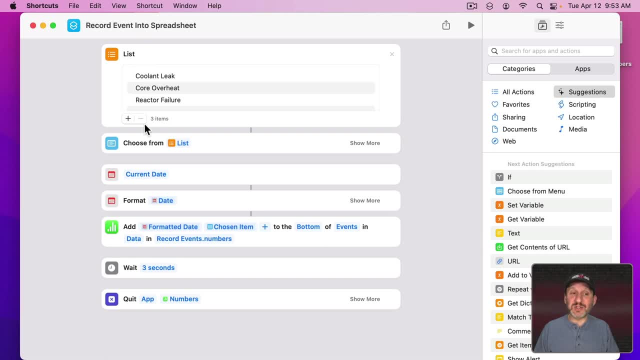 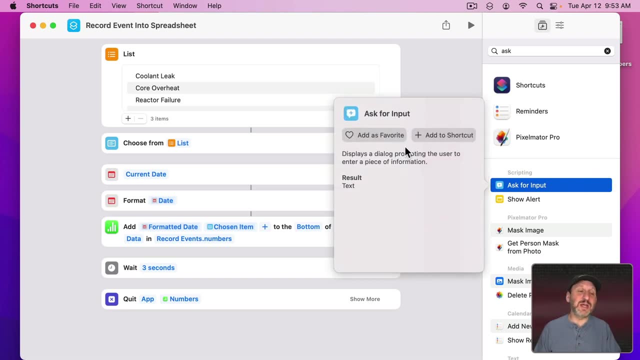 single table. in that spreadsheet You can add extra things. You can have several lists here. You can ask for input right here where you ask for a value that you can enter so you can have an item for sale, the amount sold, the total price prompt. for all of that, It automatically puts the date and 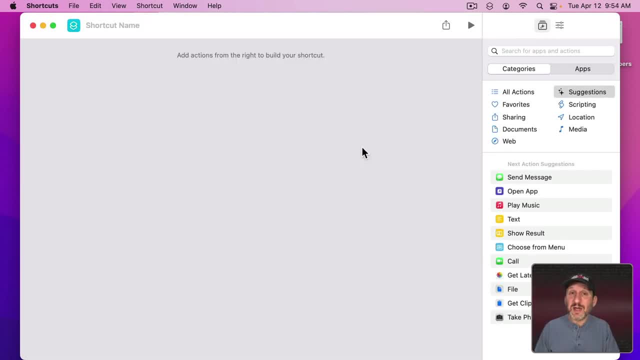 a line in a spreadsheet. Now, while those actions are new to shortcuts for a while, we've been able to use scripting to add or modify data in a spreadsheet. So there's no way to use those actions to change the value of a cell, But you could use the same scripting that you would have. 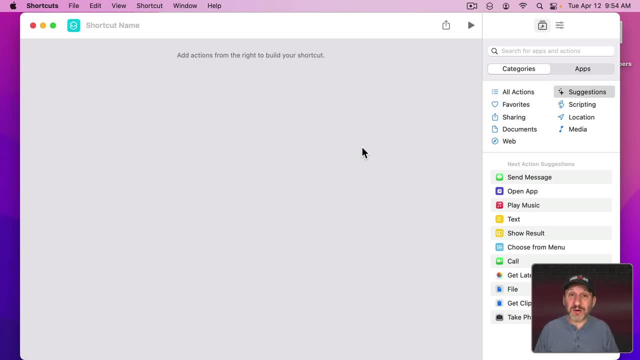 used before in shortcuts or even before shortcuts existed in Automator to change the value in the cell. So for instance, let's start off a new shortcut here by opening the spreadsheet and we'll choose that same spreadsheet right here. Let's go and say we want to change the value of